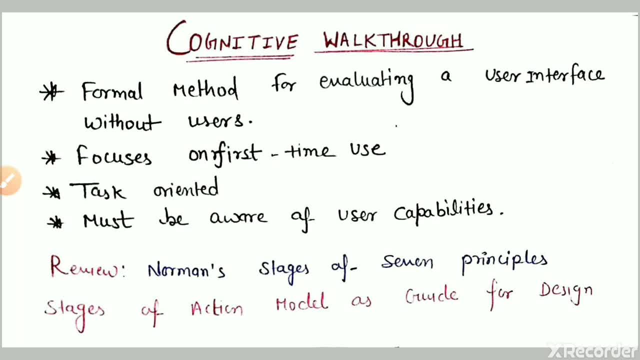 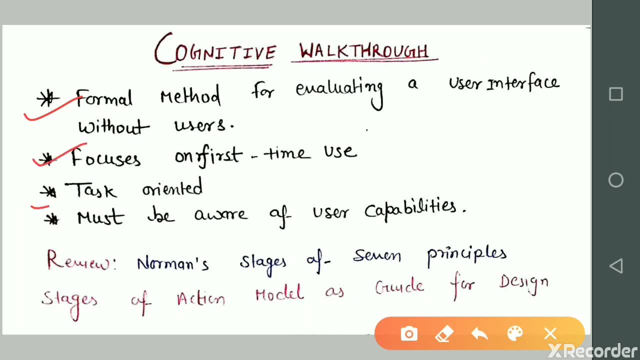 This is the formal method for evaluating user interface without user, And then it focused on the first time use And this is the task oriented And must be aware of user capabilities. And then we have review. Review is depends on normal cycle I have discussed in the previous. 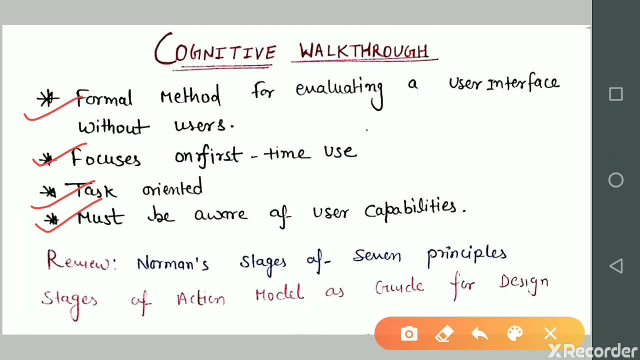 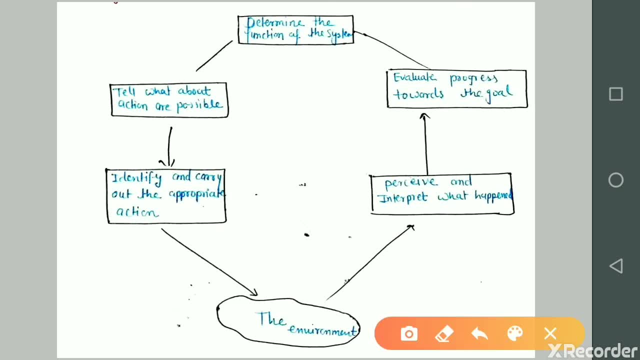 lecture number 9.. So you can see Stage of actions models as guide for design. This is the model. So first determine the function, Then what action are possible for the particular function And then identify a particular action After. 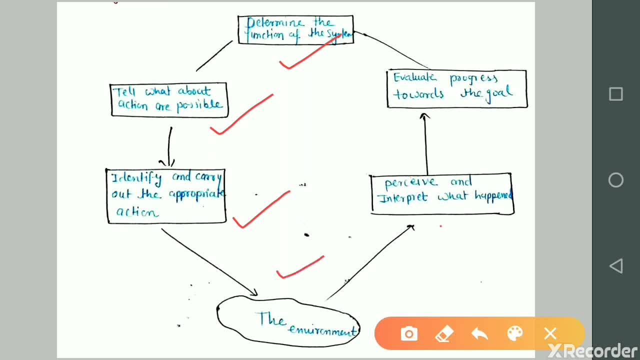 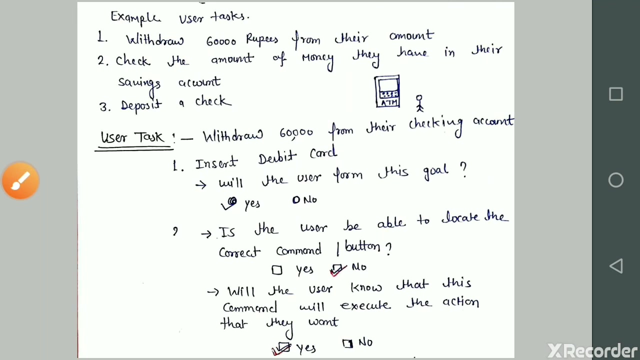 that set environment And then perceive the interpret what happen when you create a action. Last is evaluate the progress towards the goal We have already discussed in the normans principle cycle. You can see my lecture number 9.. And then We have example of ATM machine Interact a user with the ATM. So this is a ATM and this 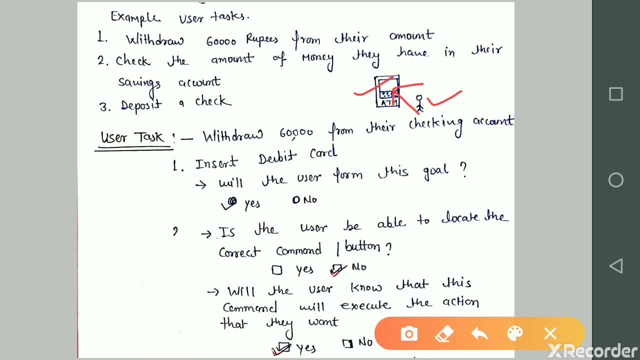 is a user And user interact with the machine. And then we have three tasks to interact with the ATM machine. First is withdraw, Withdraw 60000 rupees from their amount And then check the amount of money they have in their saving account. 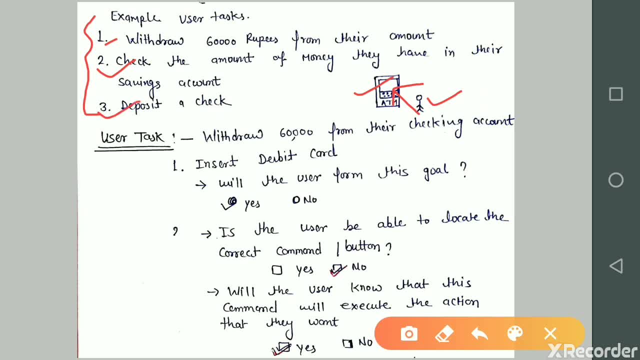 And last one is deposit a check. So these are the task After that first task of the user is withdraw money, So how we can withdraw money from the ATM machine. So what is the first is starting process: Withdraw 60 thousand from their checking account, First insert. 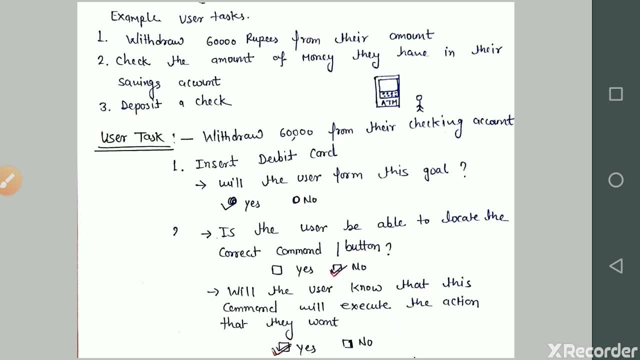 First insert debit card. will the user form this goal? If yes, is the user be able to locate the correct command? If yes or no, select according to user. and then third question is: will the user know that this command will execute the action that they want? 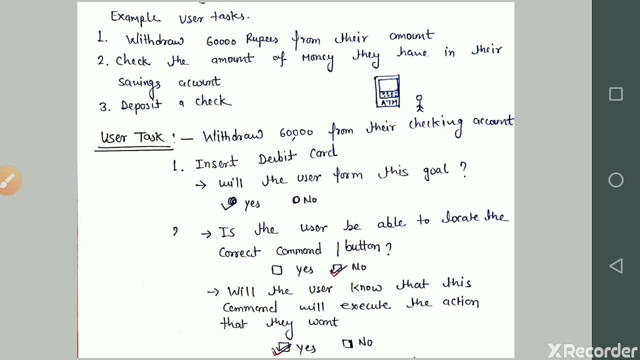 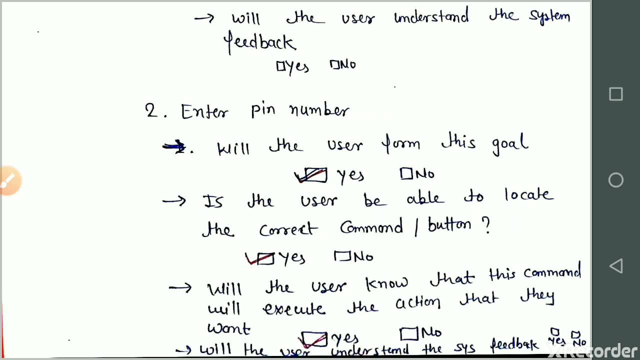 If yes or no according to user. After that will the user understand the action, give feedback? yes or no depends on user. And second task according to the user is enter PIN number. will the user form this goal? Yes, 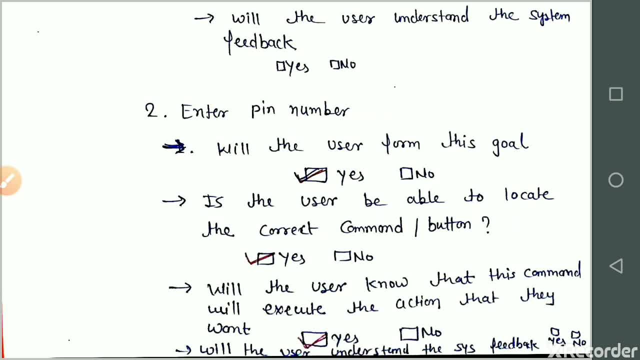 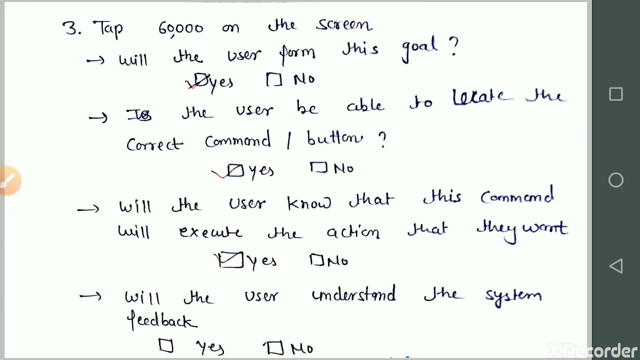 Is the user be able to locate the correct command button? If yes, will the user know that this command will execute the action that they want? If yes, will the user understand the system feedback? If yes or no, The third task is tap 60,000 rupees on the screen. will the user form this goal? 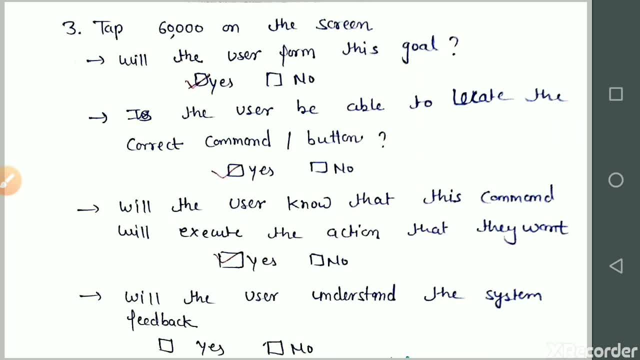 If yes, is the user be able to locate the correct command button? And if yes, will the user know that this command will execute the action that they want? If yes, will the user understand the system feedback? yes or no, they can collect money or they can't be collect the money. these are the 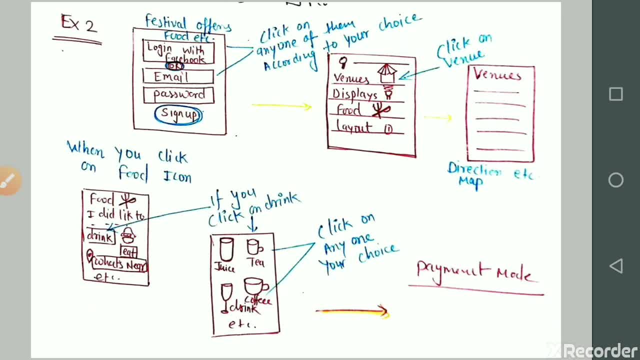 tasks. now we can take another example of if you are using net and suddenly you saw a ad on your screen that is festival offer foods. so, first of all, what you do, click on anyone from them according to the choice, like you can log in with Facebook, or you can log in with Gmail and select anyone from them. 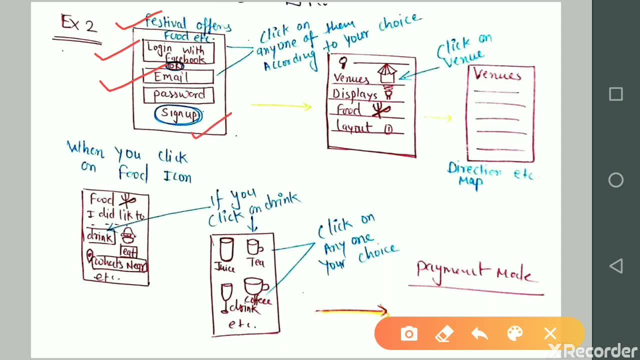 and then you can sign up. click on any one of them according to your choice. we have another window. this is a venue and this is a display. food and layout. these are the options you can choose from them. so it show you direction if you click on a venue. this 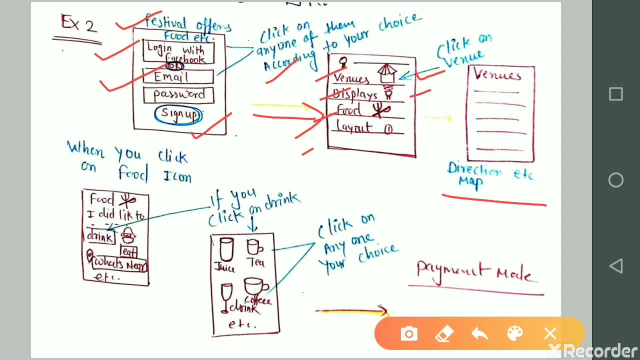 is the direction map. if you click on display, display all the all things and food or all items for eating and lay out there so many layouts according to your choice. we have different window and another window when you click on food. if you click on food, you can see the menu, what we have. have another menu and you can check.